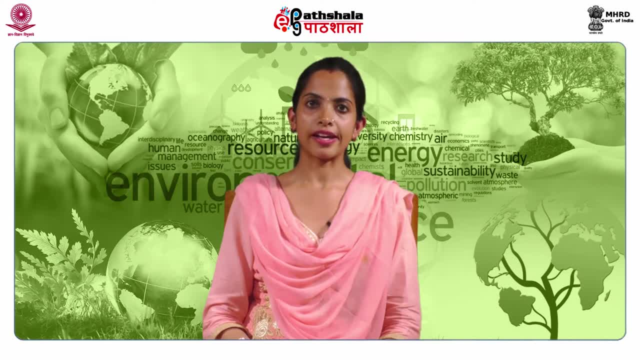 compound that exists in three phases, like solid in the form of snow, ice, hail, sleet. liquid in the form of rain water, droplets, surface ground water and gas in the form of water vapors within very short range of atmospheric temperature. 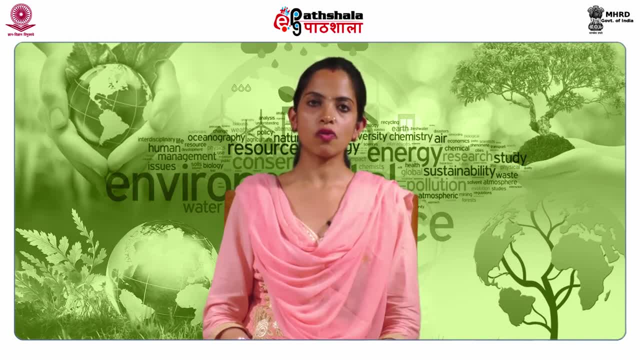 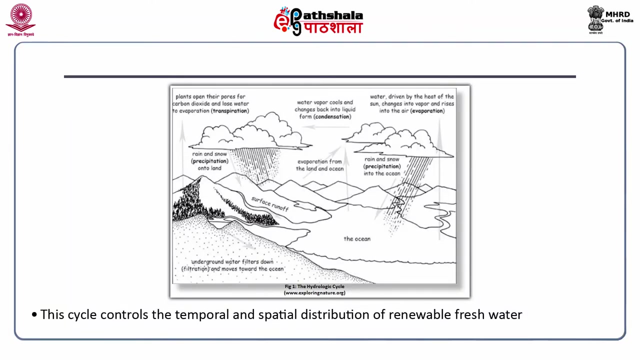 and pressure. It is the gaseous phase of water that regulates the moisture dynamics of earth and its atmosphere. There is a continuous exchange of moisture in earth and atmosphere, constituting what is called hydrological cycle, Hydrological Cycle. Hydrological Cycle: A molecule of water vapor in the atmosphere will exist in its gaseous phase for only a few days. 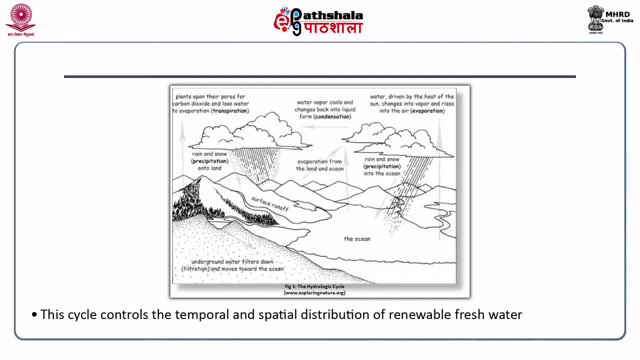 before it condenses to liquid droplets or ice crystals to form clouds or fog. Similarly, clouds and fog have limited lifespan and often evaporate away or precipitate much of their moisture within a few hours of their formation. Most of the earth's water sources 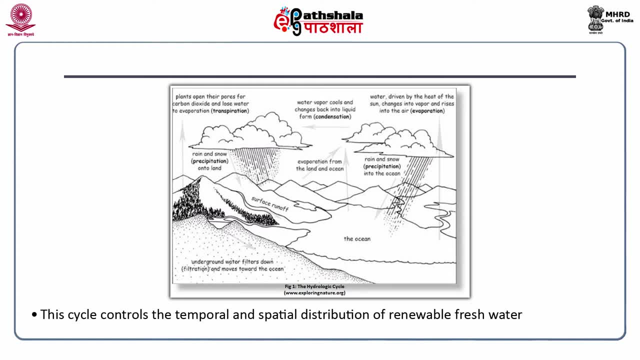 get their water supplies from this precipitation. This cycle controls the temporal and spatial distribution of renewable fresh water in the form of evapotranspiration, precipitation and runoff. Climatic factors and changes in climate further complicate the predictability of this distribution. 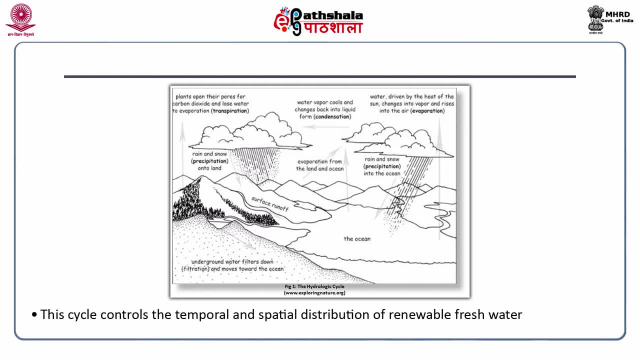 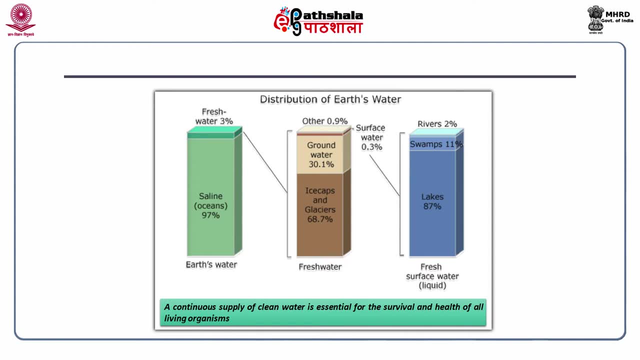 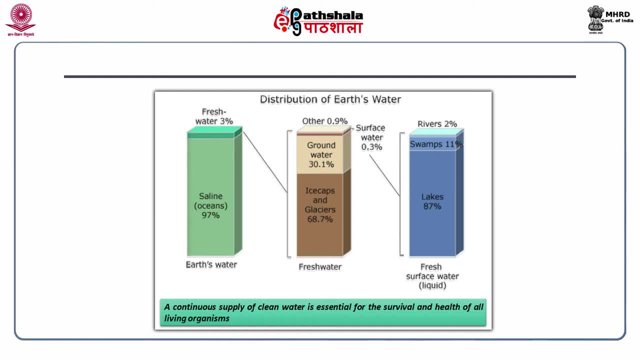 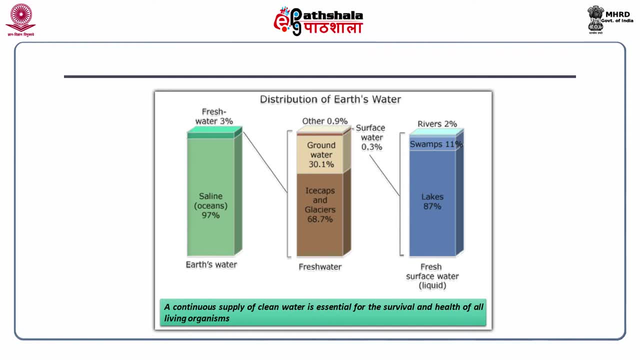 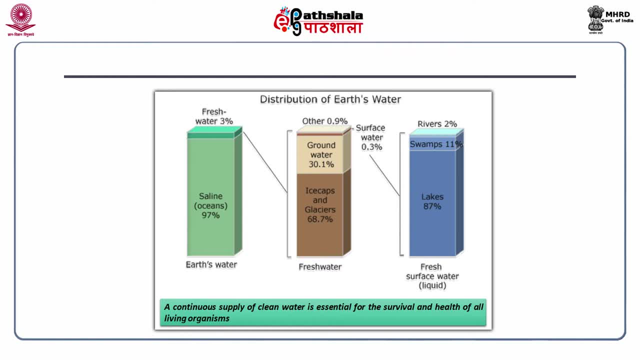 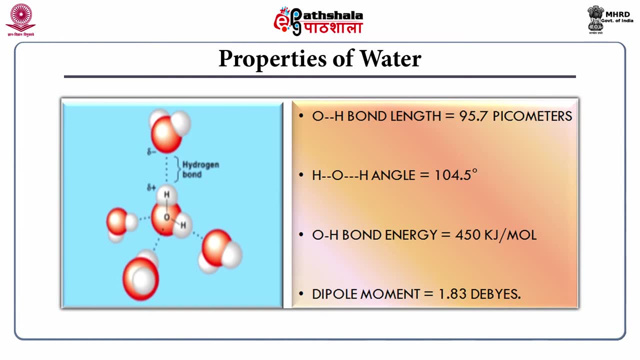 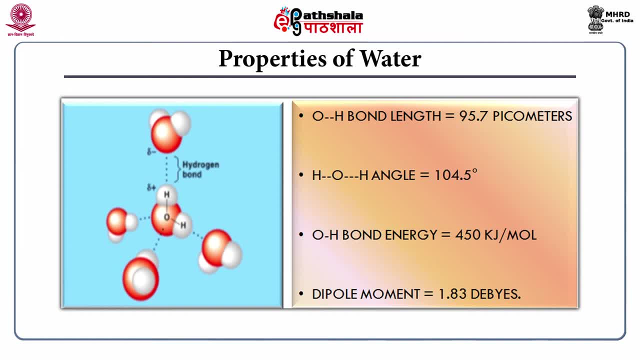 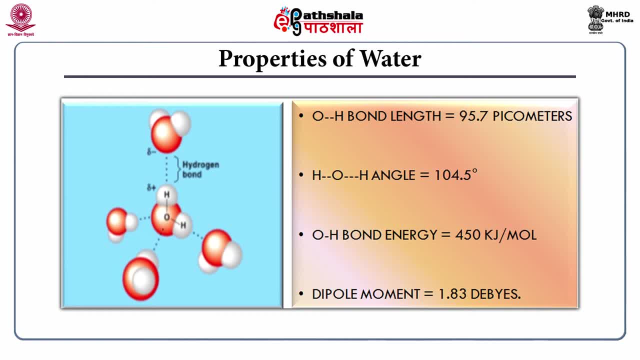 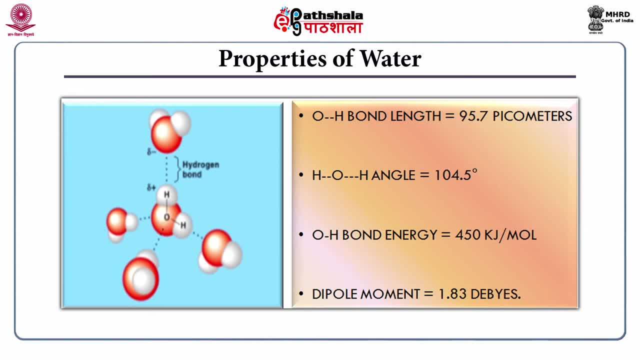 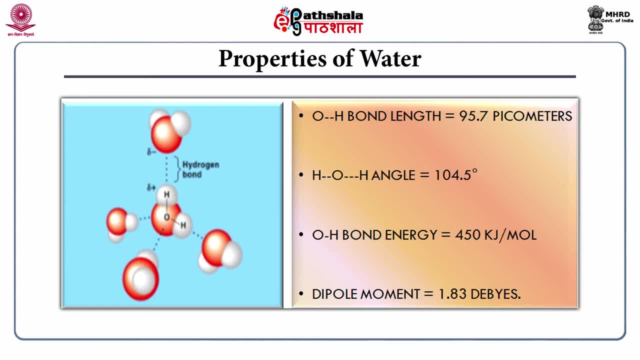 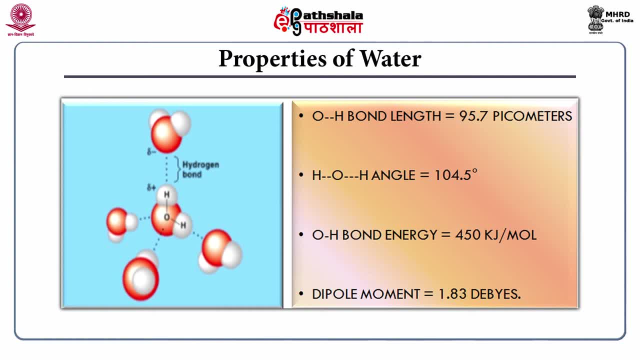 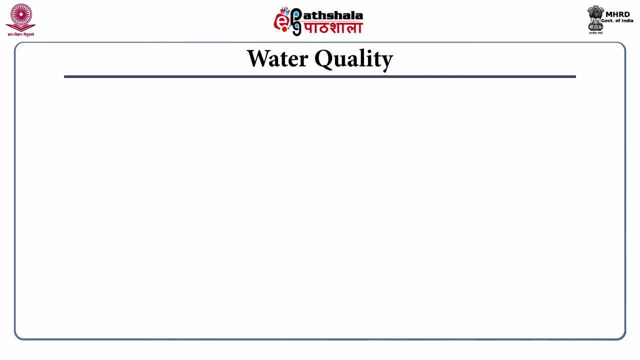 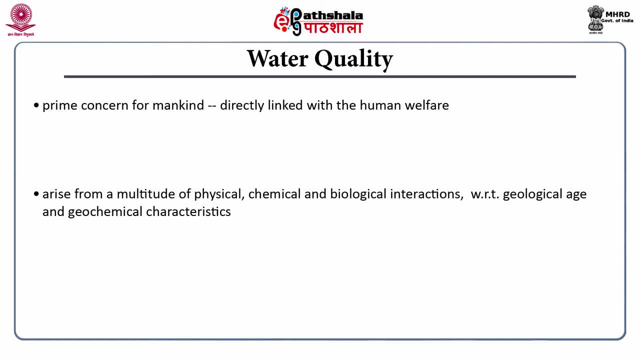 with respect to their geological age and geochemical characteristics. water quality refers to the basic physical, chemical and biological characteristics of water that determine its suitability for life or for human uses. the acceptable quality of water varies with its intended use. the characteristics of water can be classified into three broad categories. 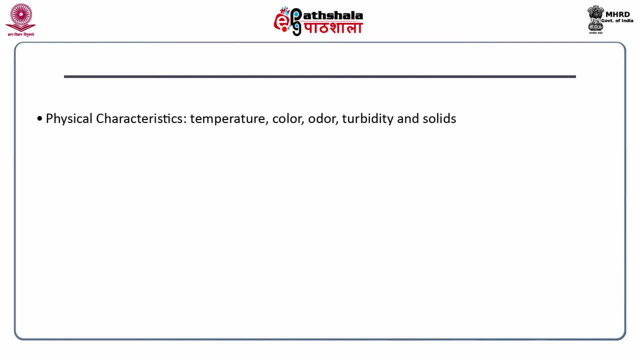 the first is the water quality and the second is the quality. the quality of water is. the quality of water? First is physical characteristics, including temperature, colour order, turbidity and solids. Second, the chemical characteristics, which include pH, conductivity, salinity, hardness. 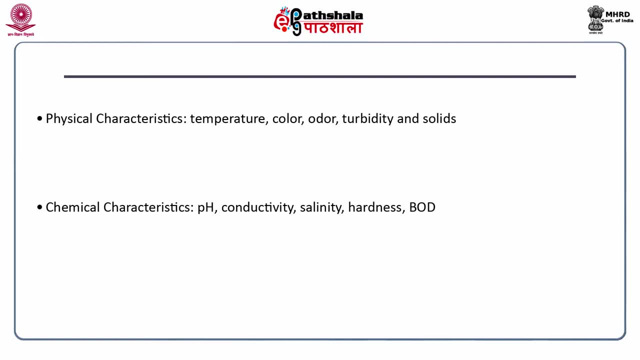 DOD, etc. and the third is biological characteristics, which accounts for counts of specific organisms and group of organisms. Let us first discuss about the physical characteristics of water. The physical characteristics are determined by sense of touch, sight, smell and taste. For example, temperature by touch, colour, floating debris, turbidity and suspended solids. 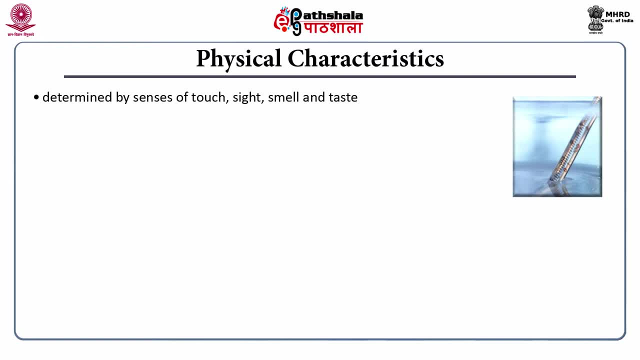 by sight and order by smell. The first characteristic is temperature, which is a measure of kinetic energy of water molecules. It is measured on a linear scale of degree Celsius or degree Fahrenheit, and it varies with the range of 10 to 21 degree Celsius, with an average of 16 degree Celsius, and depends 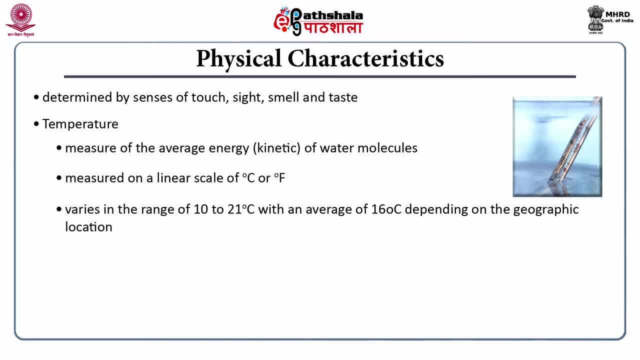 on the geographic location of the water body. Temperature affects a number of water quality parameters such as dissolved oxygen, which is a chemical characteristic. Oxygen solubility is a chemical characteristic. Oxygen solubility is a chemical characteristic. Oxygen solubility is less in warm water than the cold water. 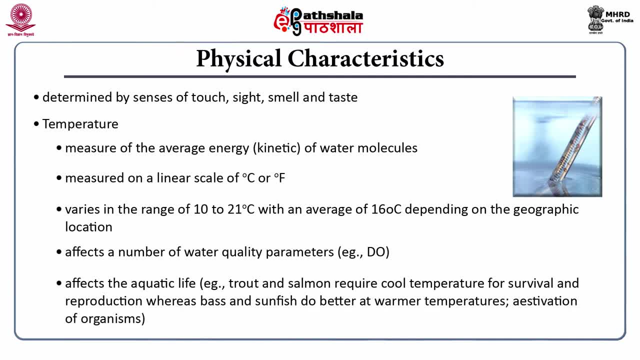 Temperature also affects the aquatic life, For example trout and salmon. they require cool temperature for survival and reproduction, whereas bass and sunfish do better at warmer temperatures. It influences the amount of oxygen that can be dissolved in water, rate of photosynthesis by alga and other aquatic organisms. 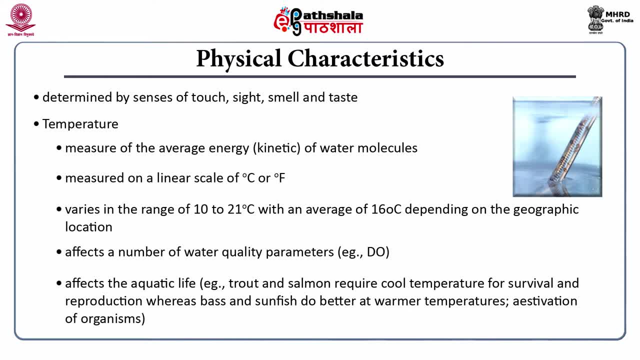 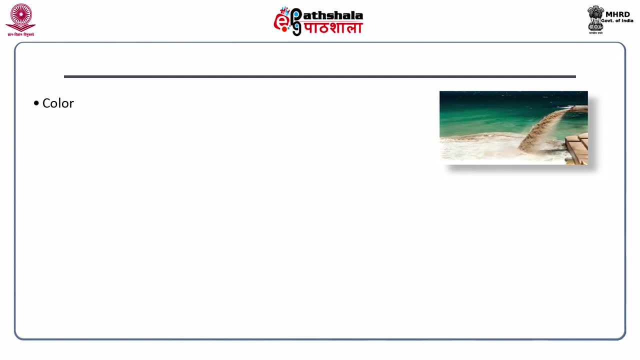 What is having Happy X-ray matches or not to were. Formal examination of right anatomy has often been combined with risk assessment In 4 versions of thecc. Baby mice can be 콩 prepare in ağe ized water to eat graftier. 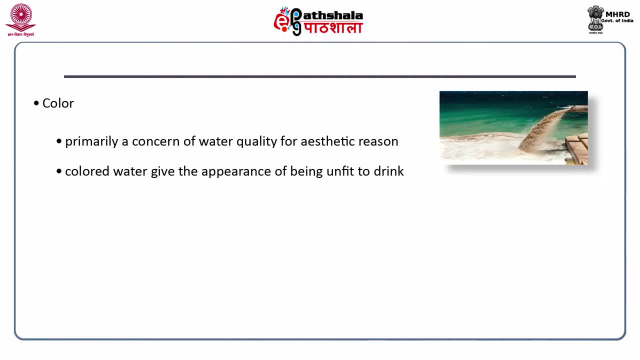 Algae of stale food communities can disappear due to disappear all deadаний, All aware of mould up to in conocer vo timers, thesemittles and other aquatic plants. metabolic though the water may be perfectly safe for public use, Color of water body can indicate the presence of organic substances such as algae or humic. 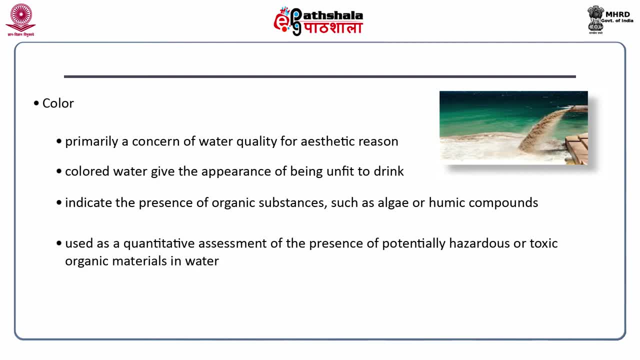 compounds. In recent times, color has been used as a quantitative assessment of the presence of potentially hazardous or toxic organic materials in water. Determination of color can help in estimating the costs which are related to discoloration of water. It is reduced or removed from the water through the use of coagulation, settling and filtration. 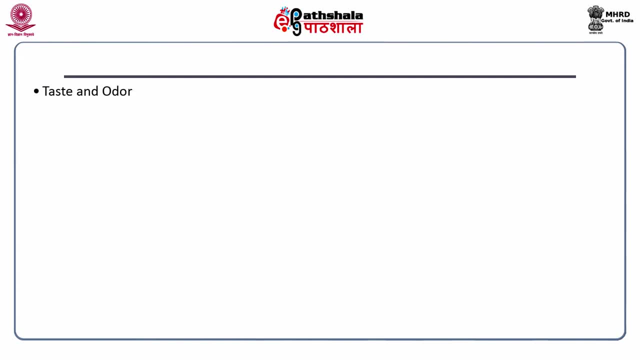 techniques, Taste and order-. These are basically the human perceptions of water quality. Human perception of taste includes sour like hydrochloric acid, salty like sodium chloride, sweet like sucrose and bitter like caffeine. Simple compounds relatively produce sour and salty taste. 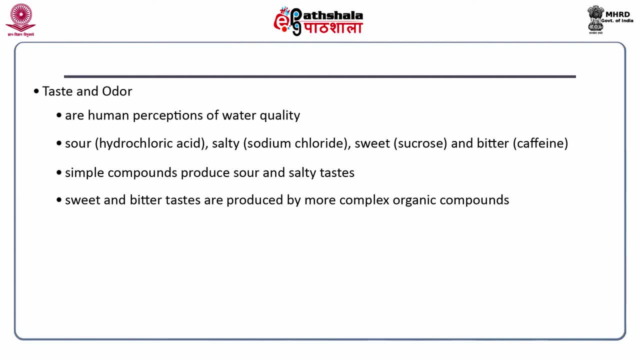 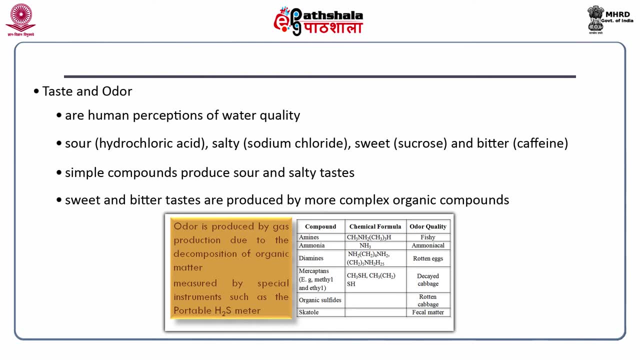 However, sweet and bitter tastes are produced by more complex organic compounds. Order in water is produced by gas production due to the decomposition of organic matter or by substances added to the wastewater. It is measured by special instruments such as potable hydrogen sulphide mixtures. 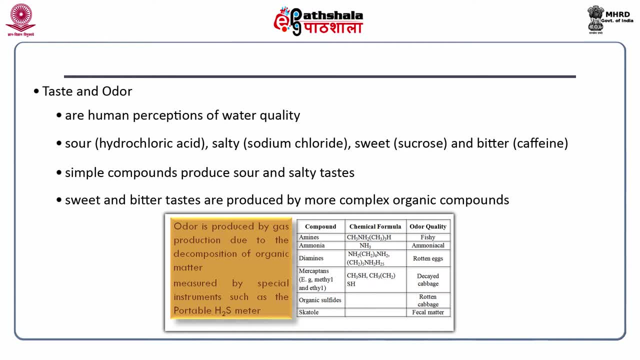 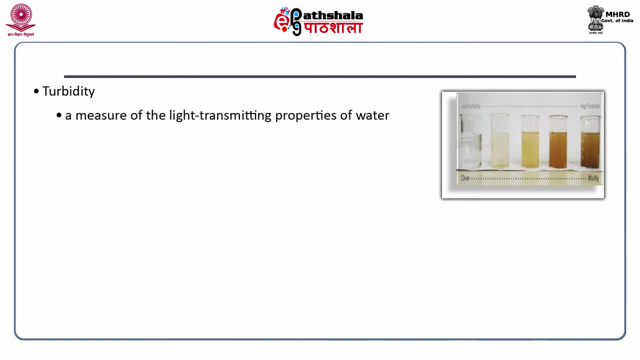 Hydrogen sulphide meter, which is used for measuring the concentration of hydrogen sulphide. Some examples of order producing substances are amines, ammonia, diamines, mercaptanes, organic sulphides and scatoles. Next characteristic is turbidity, which is basically a measure of light transmitting. 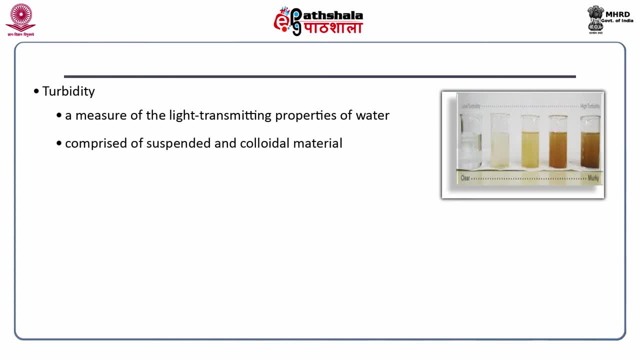 properties of water and is comprised of suspended and colloidal material. It is important for health and aesthetic reasons. Transparency of natural water body is affected by human activity, decaying plant matter, algal blooms, suspended sediments and plant nutrients. Turbidity provides an inexpensive estimate of total suspended solids concentration. 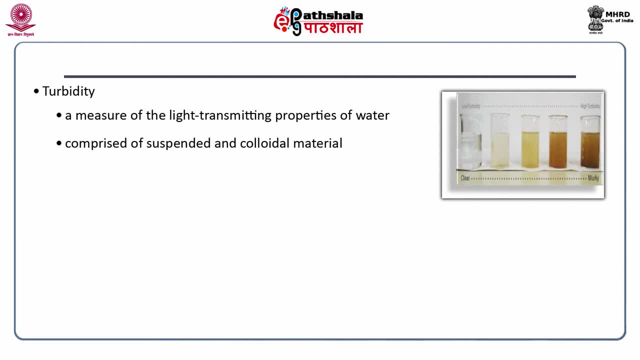 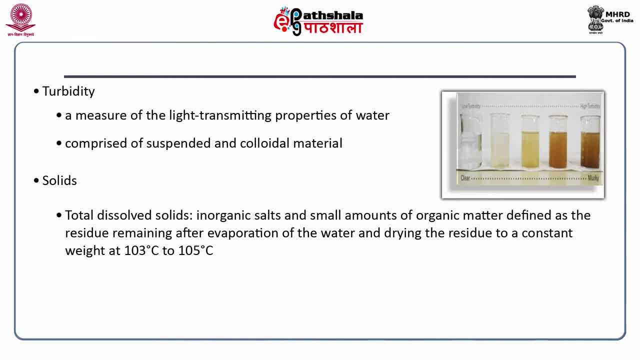 The TDS content of water is defined as the residue remaining after evaporation of the water and drying the residue to a constant weight as 103 carotene CO2 vs 105 carotene CO2.. CE será modificado. Constituents of TDS are usually calcium, magnesium, sodium and potassium cations and carbonate, bicarbonate, chloride, sulfate and nitrate anions. 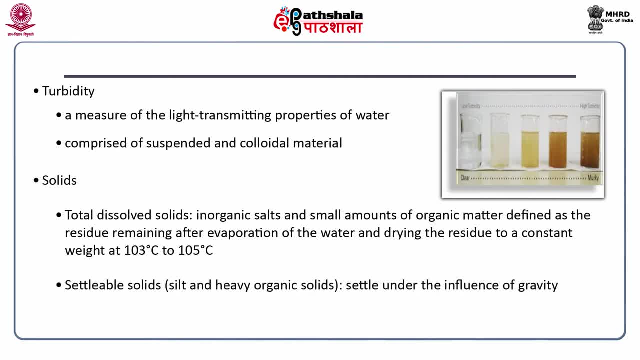 Satellable solids, ie silt and heavy organic solids, are those that settle under the influence of gravity. However, suspended solids are classified based on particle size and retention of these on standard glass fiber filters. The significance of suspended solids in water is great on a number of grounds. 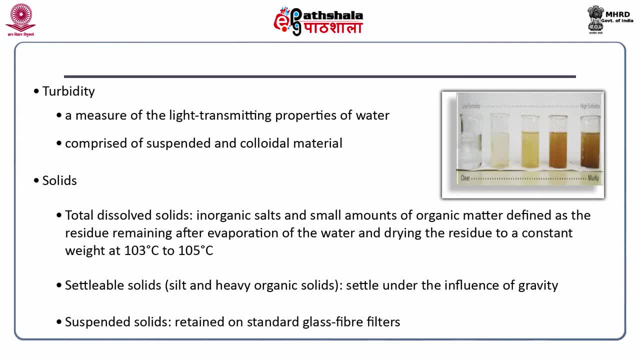 The solids may in fact consist of algal growths, leading to severe eutrophic conditions in any water body. Deposition of these on bed of rivers and lakes may give rise to septic and offensive conditions, and they may indicate the presence of unsatisfactory sewage effluent discharges. 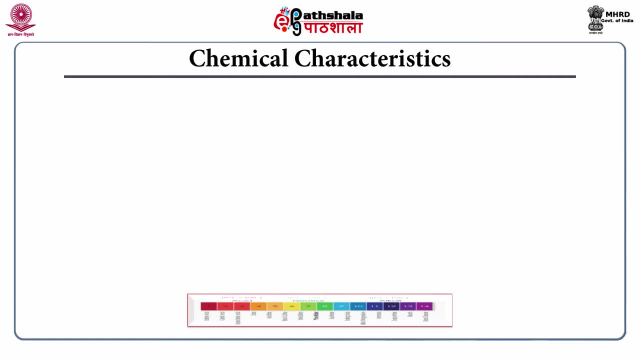 Now we will discuss about the chemical characteristics of water. The health concerns which are associated with chemical constituents of drinking water arise mainly from their ability to cause adverse health effects. There are few chemical constituents of water that can lead to health problems resulting from even a single exposure. 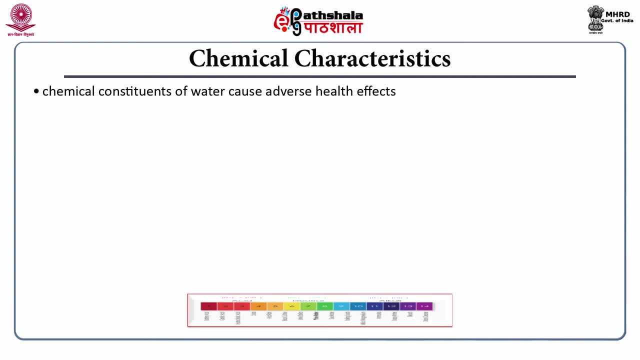 An appreciable number of serious health concerns may occur as a result of chemical contamination of drinking water. The major chemical properties of the water are now being discussed, And the first one is pH, which is a negative log of hydrogen ion concentration. It is actually a measure of how acidic or basic the water is. 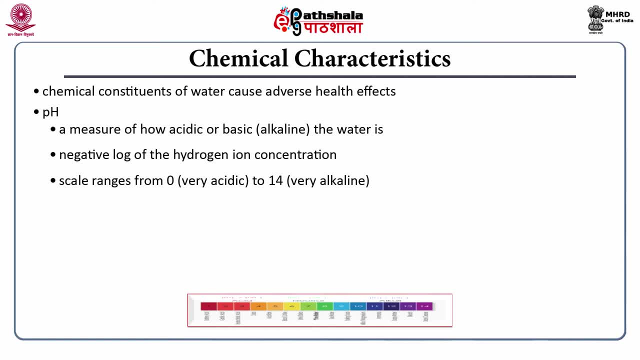 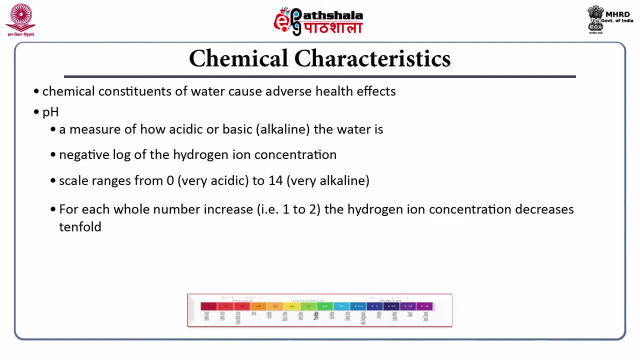 to 14 for very alkaline water to 14 for very alkaline water, to 14 for very alkaline water. For each hole, number increase the hydrogen ion concentration decreases tenfold and the water becomes less acidic. The most frequently encountered range of pH of fresh water is 6.5 to 8.. 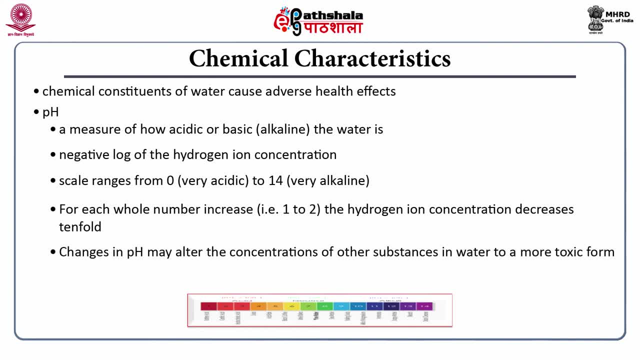 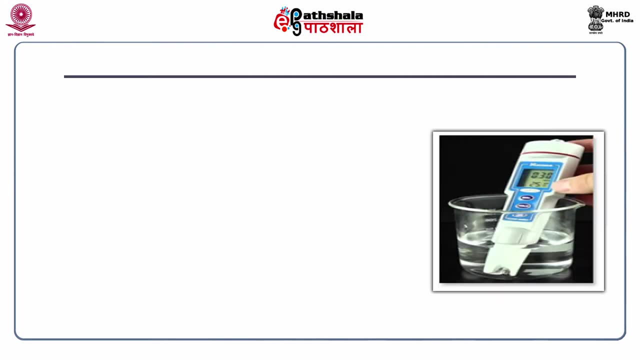 Changes in pH may alter the concentration of other substances in water to a more toxic form. Ammonia toxicity, chlorine, disinfection efficiency and metal solubility: all are subjective to changes in pH value. Electrical conductivity is basically the ability of water to conduct an electric current as 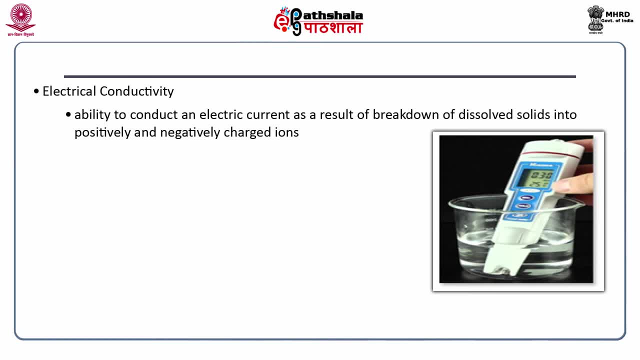 a result of breakdown of dissolved solids into positively and negatively charged. The major positively charged ions include potassium, sodium, calcium and magnesium. The major negatively charged ions in water are chloride, sulphate carbonate and bicarbonate. Nitrates and phosphates are the minor contributors to electrical conductivity, although they are 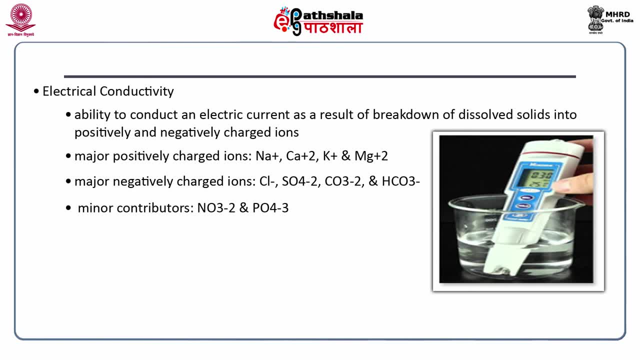 very important biologically. Conductivity will vary with the water source, ie ground water, water drained from agricultural fields, waste water, rainfall. therefore, conductivity can indicate groundwater seepage or sewage leak. the next characteristic is salinity, which is a measure of the amount of salts in the water, because 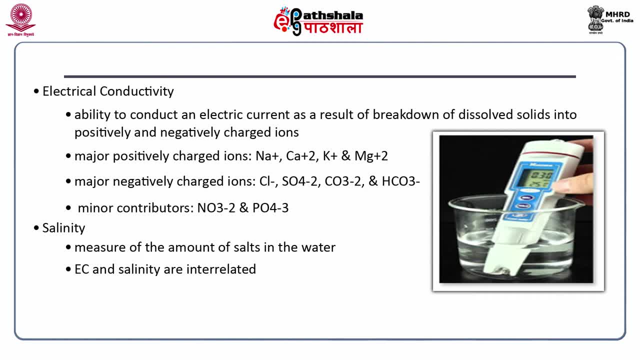 dissolved ions increase salinity as well as conductivity of any solution. the two measures are interrelated. salt affect the quality of water used for irrigation or drinking purpose. they also have a critical influence on aquatic biota, as every kind of organism has a typical salinity range and type of salt that it can tolerate. for example, Cladocerans, the water flares are. 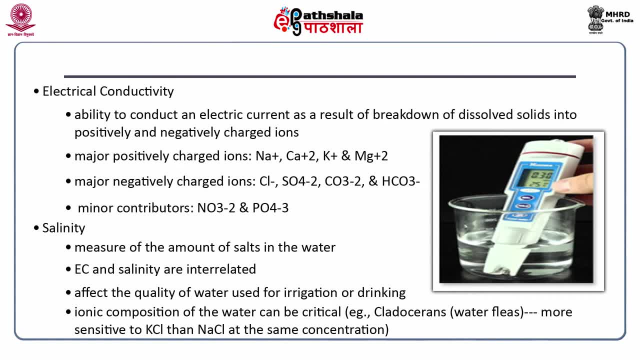 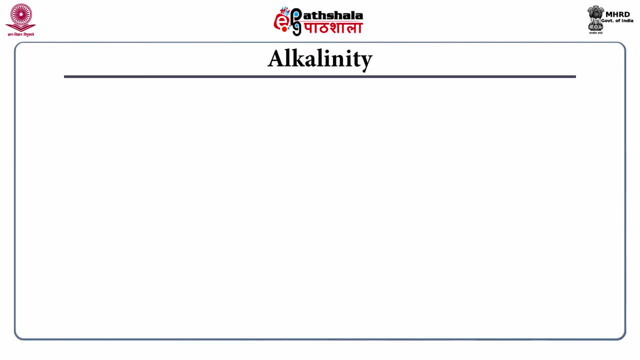 far more sensitive to potassium chloride then sodium chloride at the same concentration. the alkalinity of natural water is a measure of the capacity of water to neutralize essence and thereby it reflects its buffer capacity. it is generally attributed to the presence of bicarbonates, carbonates and hydroxides. alkalinity is important for fish and aquatic life because the 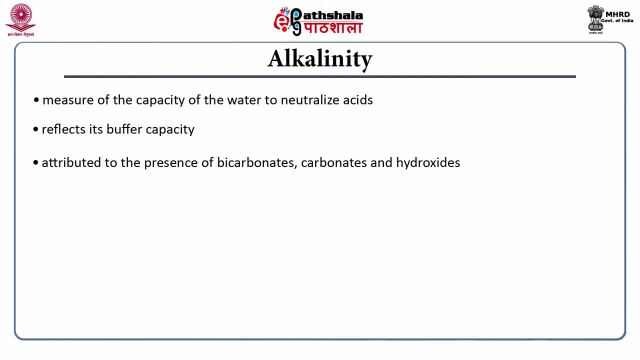 function best in a range of 6 to 9 pH. alkalinity in streams in is influenced by rocks and soils, salts, certain plant activities, industrial waste water discharges. oligotrophic lakes with low nutrient content tend to have lower alkalinity, while eutrophic lakes with high nutrient levels have a tendency of higher alkalinity when a 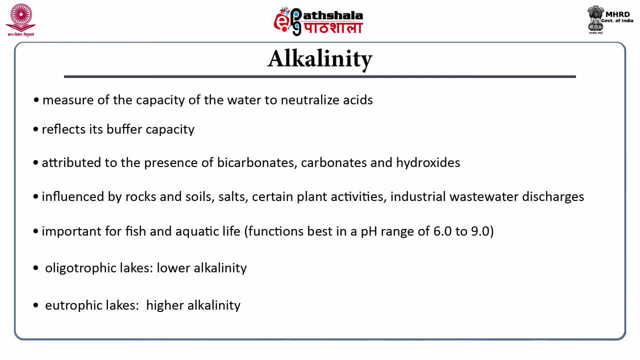 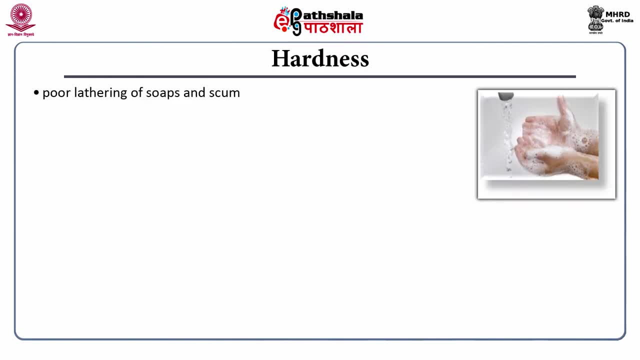 water sample is observed to be producing poor leather with soap and scum. it is said to be hard water. hardness is the natural characteristic of water, which can enhance its palatability and consumer exceptibility for drinking purposes. the hardness of water is due to the presence of calcium and magnesium, minerals that are naturally present in the water. 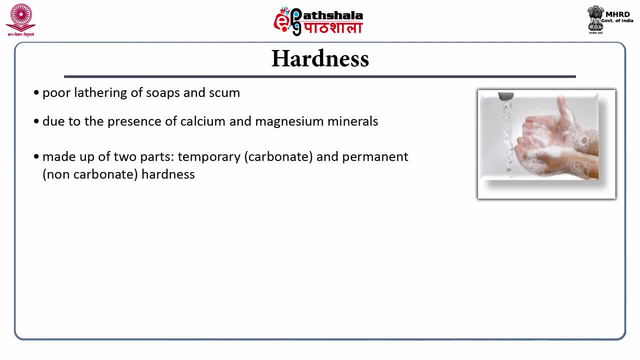 the hardness is made up of two parts: temporary, the carbonate hardness, and permanent, the noncarbonate hardness. the temporary hardness of water can easily be removed by boiling the water. hardness is expressed in milligram per liter. as calcium carbonate, the water is said to be strong as calcium may be present in tank�GR. 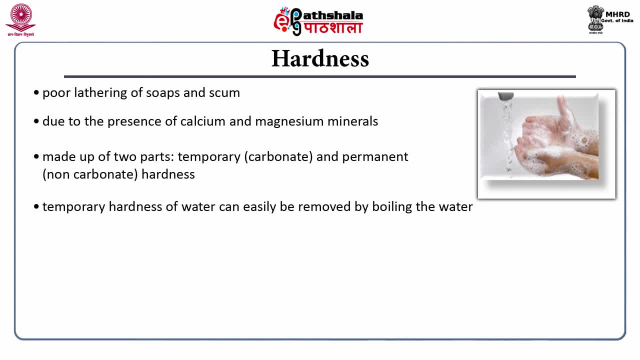 in mg per litre as calcium carbonate. the water is said to be soft if it has hardness in the range of 0 to 100 mg per litre as calcium carbonate, moderate if the range is between 100 to 200 mg per litre as calcium carbonate, and so on. The extremely hard water has a range of hardness. 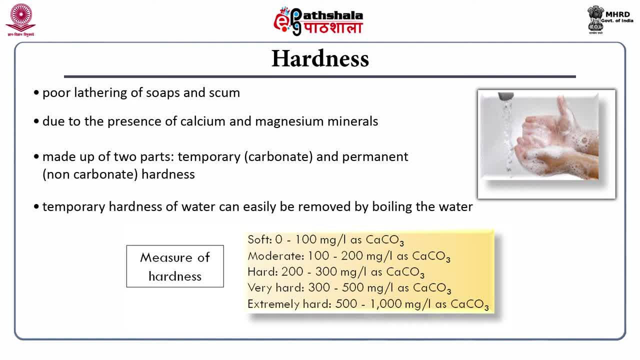 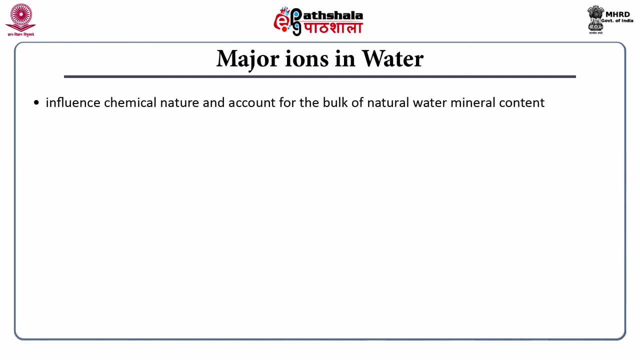 falling between 500 to 1000 mg per litre as calcium carbonate. There are various kinds of trace ions in water supply that influence chemical nature and account for the bulk of natural water mineral content. Most of the dissolved inorganic chemicals in fresh water occur as ions. These ions come in water body from atmospheric deposition, rock weathering. 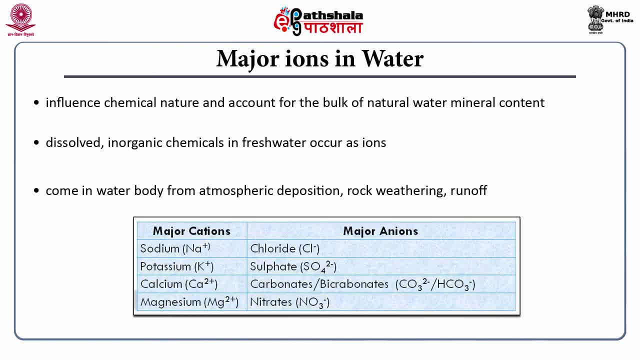 runoff, etc. The main ionic species of natural water are sodium, potassium, calcium and magnesium, and the anions constitute chlorophyll. Sodium is an essential nutrient element in drinking water supplies, but in its excessive quantities it acts as a laxative. Calcium is essential for water conserve properties in water. 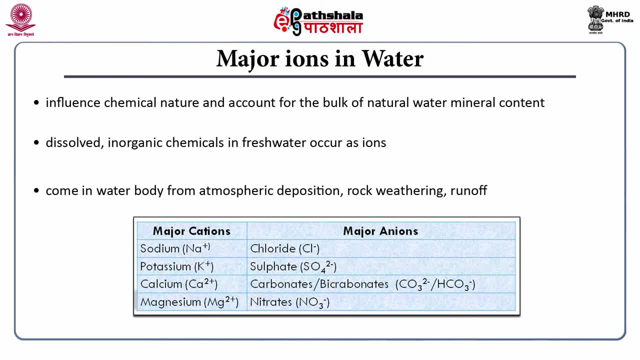 drugs and hot water processesarticles. Raspberry waterское is called cor, parade is called hundred. Essential to human nutrition, are a key element in the formation of teeth and bones. It is also known as limestone and is a cause of water hardness. Magnesium is one of the most common elements in the earth crust. 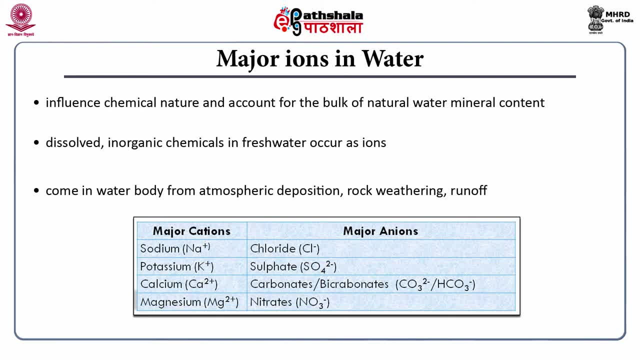 Sulfates of magnesium at very high concentrations may have laxative effect on some people. Chloride in drinking water is generally not harmful to human health, except when present in high concentration that may be injurious to heart and kidney patients. Water with objectionable sulfate content may have a bitter taste. 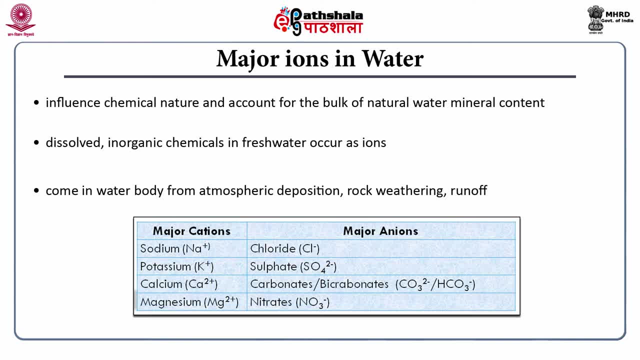 It also contributes to odor problems. Excessive bicarbonate add to salinity and total solid content of water, while carbonate content of water can also be considered as temporary water hardness Nitrates, even at low concentration, can cause health problems to infants of 6 to 12 years. 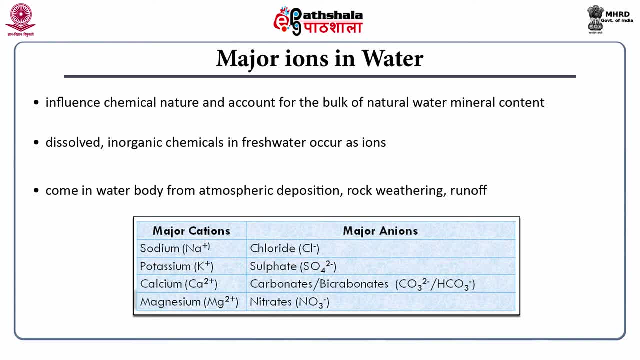 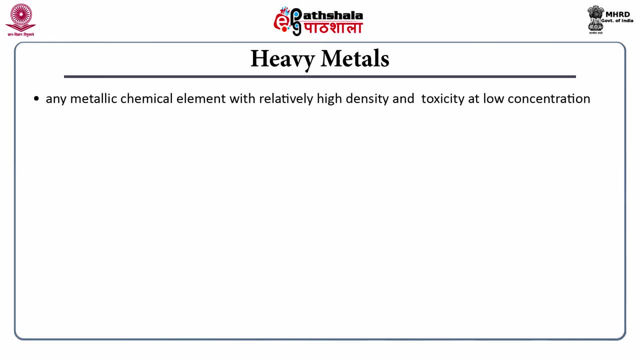 of age or less and pregnant women by affecting the oxygen carrying capacity of the blood. Heavy metal refers to any metallic chemical element that has a relatively high density and toxicity at low concentration. Some major examples of heavy metals are mercury, cadmium, arsenic, chromium, nickel, copper. 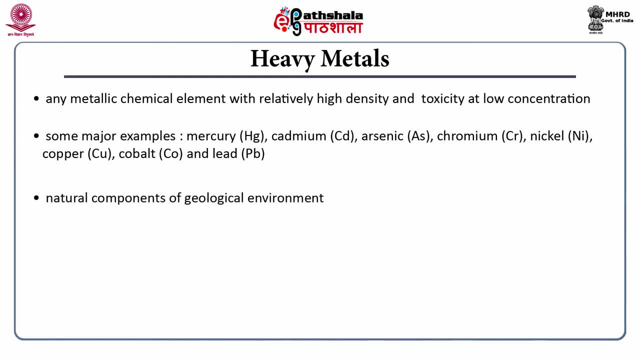 cobalt and lead. Heavy metals are basically the natural components of geological environment. They enter the human body via food, drinking water and air to small extent. Some heavy metals, for example copper, selenium, zinc, are necessary to keep up the metabolism of human body as trace elements. 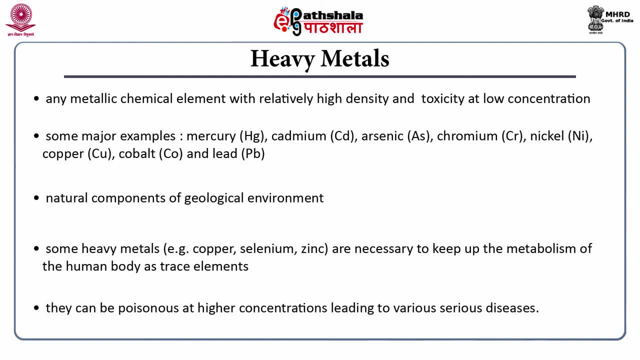 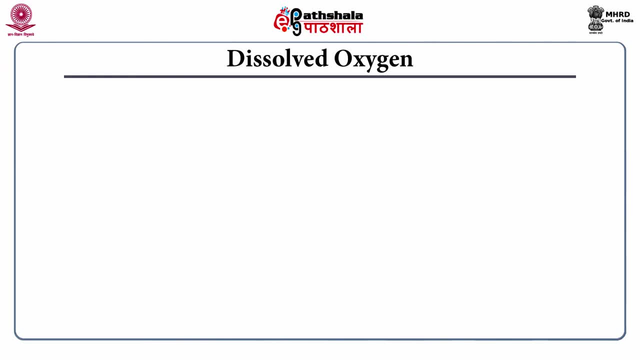 However, they can be very poisonous at higher concentrations, leading to various serious health diseases. The chemical characteristic of water with high importance is dissolved oxygen. That can be expressed as the amount of gaseous oxygen dissolved in an aqueous solution. It gets into water by diffusion from the surrounding air, by aeration, that is, rapid movement, and 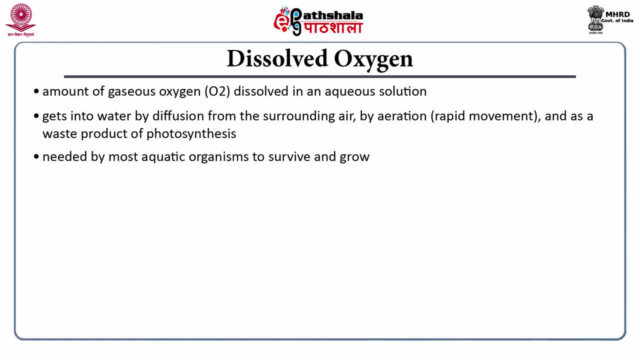 as a waste product of photosynthesis. The oxygen in dissolved form is needed by most aquatic organisms for their survival and growth. Organisms such as trout and stoneflies require high amount of dissolved oxygen, while some others, like catfish, worms, dragonflies, can survive in somewhat lower amount. 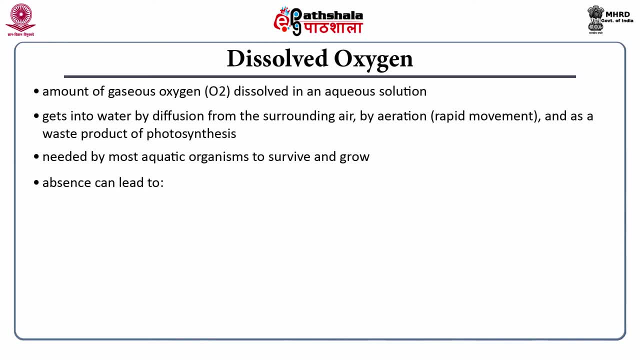 The absence of enough amount of oxygen in water can lead to deaths of adults and juveniles. reduction in growth, failure of eggs or larvae to survive. change of species present in a given water body. The hypoxic conditions in water body, ie DO when measured is less than 3 mg per litre. 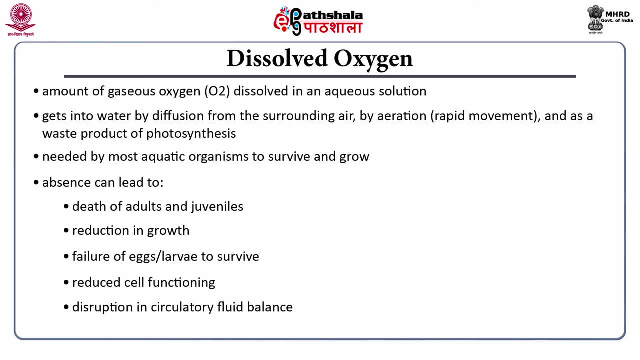 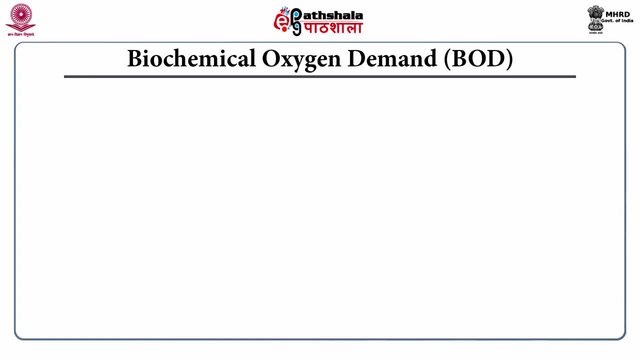 causes reduced cell functioning and destruction. This is the main reason for the lack of oxygen in water. The next important characteristic is biochemical oxygen demand, which is the amount of dissolved oxygen required by aerobic biological organisms to degrade the organic matter present in water body at certain temperature over a specific time period. 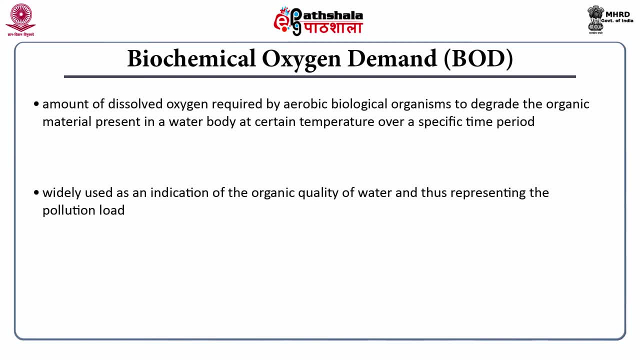 It is widely used as an indication of the organic quality of water and thus reduces the pollution load. It is most commonly expressed in mg of oxygen consumed per litre of sample during 5 days of incubation at 20°C and symbolically represented as BOD5.. 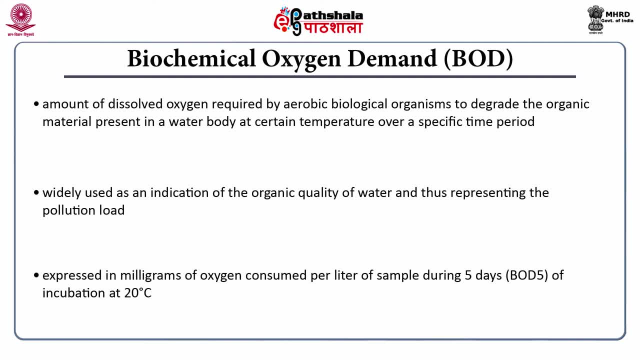 When organic matter decomposes, microorganisms such as bacteria and fungi, they feed upon this decaying material and eventually the matter becomes oxidised. The harder the microorganism decomposes, the harder the material becomes oxidised. The harder the microorganism decomposes, the harder the material becomes oxidised. 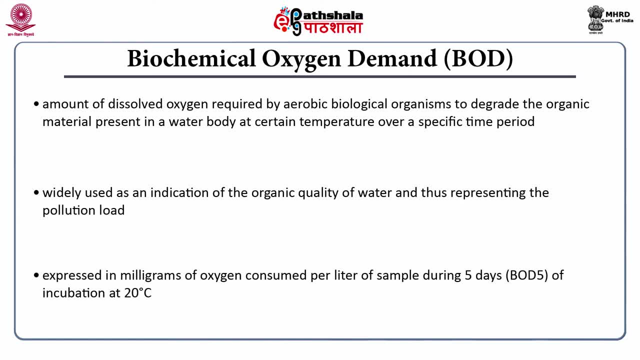 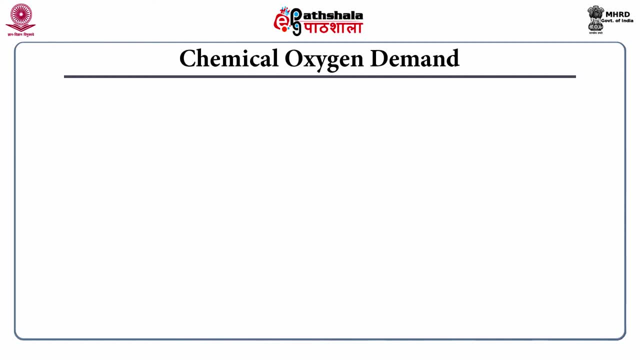 The harder the microorganism decomposes, the harder the material becomes oxidised. The time period in which the microorganisms work, the more oxygen will be used up, giving a high measure of BOD, leaving less oxygen for other life in water. Chemical Oxygen demands determine the quantity of oxygen required to oxidise the organic. 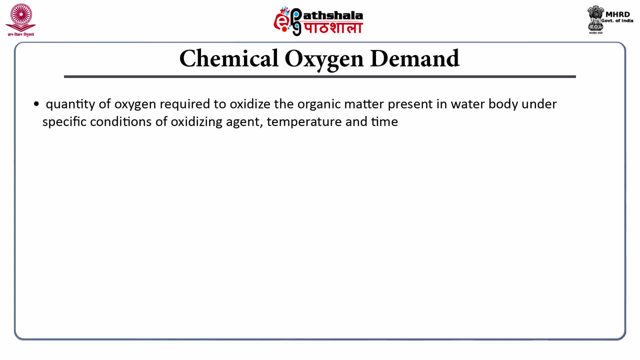 matter present in water body under specific conditions of oxidising agent, temperature and time. It is a important water quality parameter A A index to assess the effect of discharge waste water that it will have on the receiving environment. Higher COD levels represent the presence of greater amount of oxidizable organic material. 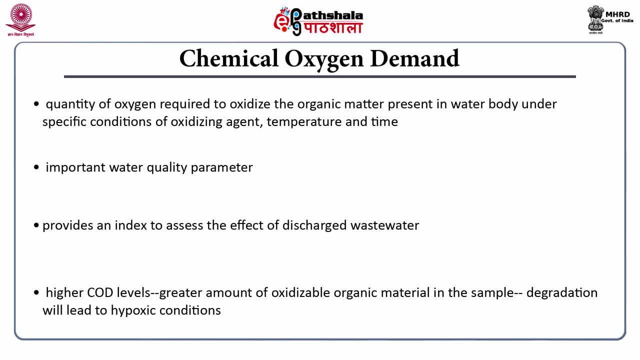 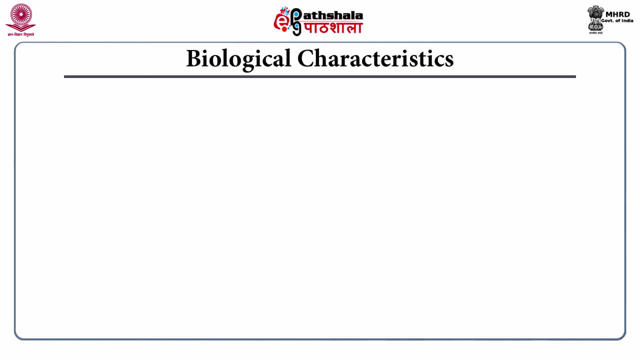 in the sample, the degradation of which eventually will again lead to hypoxic conditions in the water body. The third category of water characteristics is its biological characteristics, which includes microbial contamination and presence of fecal matter. Microbial contamination is one of the major concerns of water quality. Many types of microorganisms are naturally present in the water. 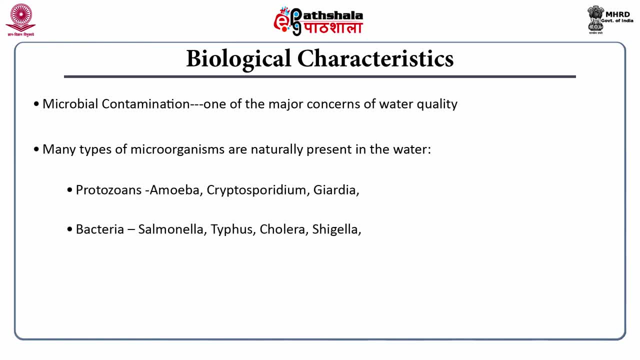 including protozoans, bacteria, viruses and helminthes. Fecal matter constitutes coliform bacteria. total coliform bacteria, fecal coliform bacteria and E coli are all considered indicators of water quality Contaminated with fecal matter. Total coliform bacteria are an entire group. 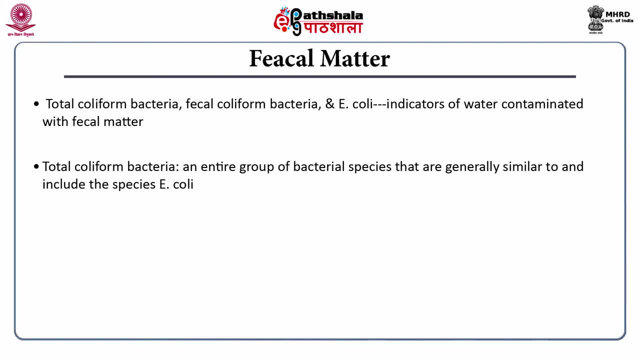 of bacterial species that are generally similar to and include the species of E coli. Fecal coliform bacteria are basically the coliform bacteria that do live in fecal matter, including, but not limited to, the species of E coli. Most of the fecal coliform cells found in 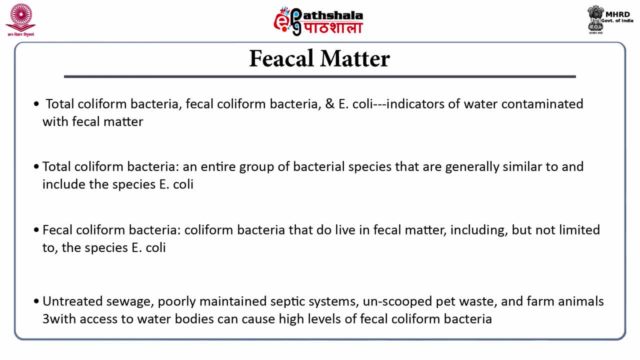 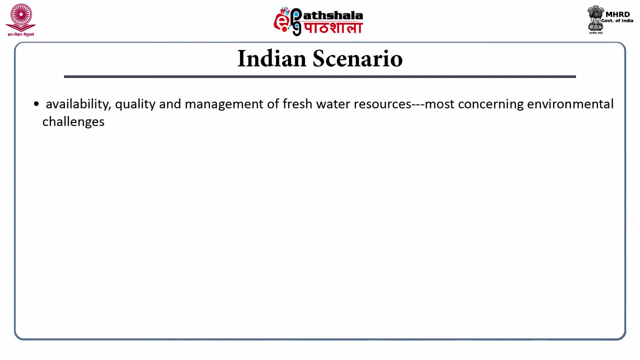 fecal matter are E coli. Untreated sewage, Poorly maintained septic systems, Un-scooped pet waste, Farm animals with excess to water bodies can cause high levels of fecal coliform bacteria to appear in and make the water unhealthy. If we talk about Indian scenario, the availability, quality and management of fresh water resources. 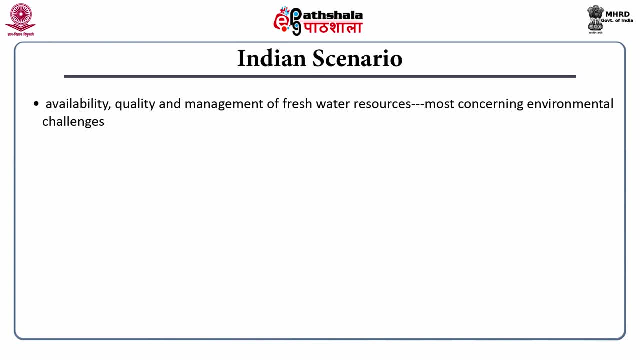 is one of the most concerning environmental challenges of national importance in India. To overcome these challenges, we need to understand the importance of water quality. The importance of water quality is one of the most important challenges of national importance in India. CPCB, the Central Pollution Control boards of Government of India, is playing a pivotal 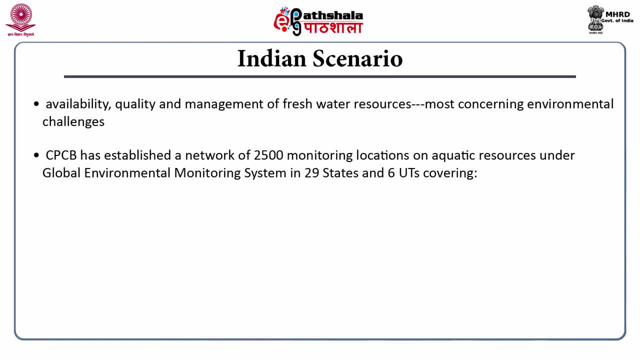 role. CPCB has established a network of 2,500 monitoring locations covering 445 rivers, 154 lakes, 12 tanks, 78 ponds, 41 creeks or sea water, 25 canals, 45 drains, 10 water treatment plants. 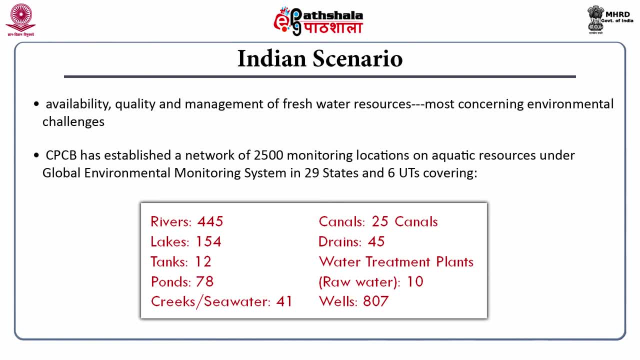 and 807 wells across the country under global environmental monitoring systems. Not only are they covering all the important areas of the country, but they are also having to monitor the statewide water quality of the places they are all connected to. There are plenty of water quality products. 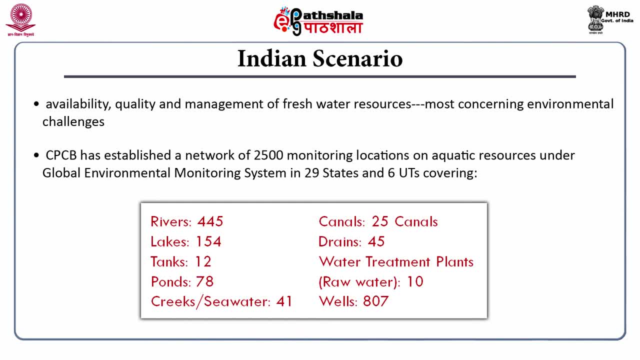 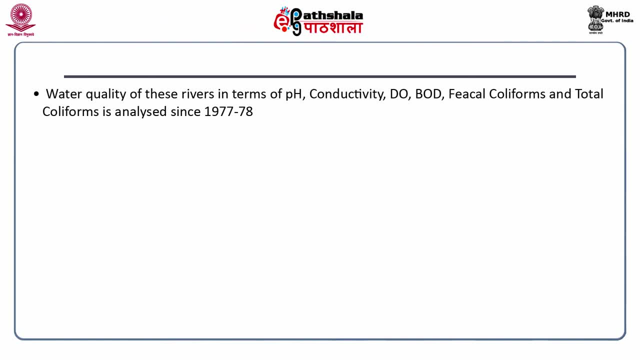 monitoring system in 29 states and 6 union territories. Water quality of these rivers in terms of pH, conductivity, dissolved oxygen, biological oxygen demand, fecal coliforms and total coliforms is analyzed since 1977-78.. The various reports published by CPCB till now: 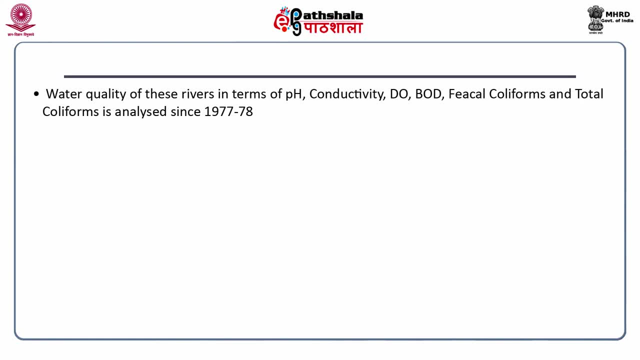 indicated that BOD and coliforms continue to be the major water quality issues. The board has identified 302 polluted river stretches on 275 rivers in 27 states and 2 UTs on the basis of BOD level and has prioritized them. Out of these 302 polluted stretches, 34 in class 1 ie- BOD. 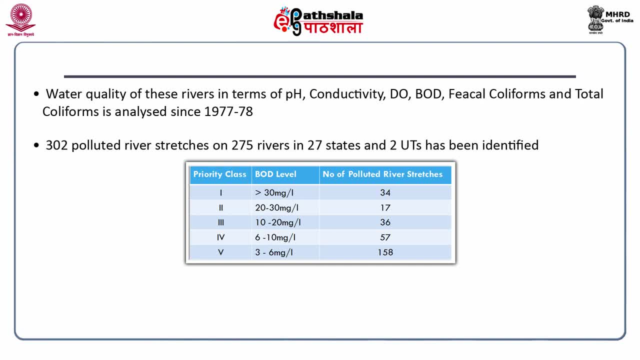 greater than 30. The maximum number of polluted river stretches were observed in the state of Maharashtra, with 49 sampling points. The only river of Delhi, ie Yamuna, is under priority class 1, a pathetic and alarming situation. So a large number of water bodies were.